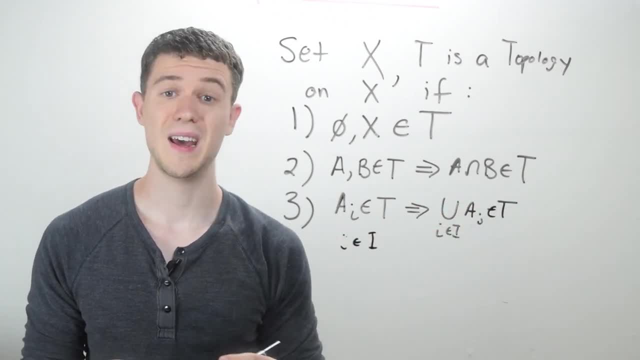 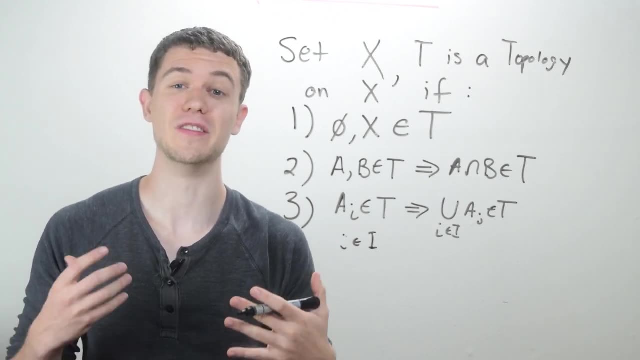 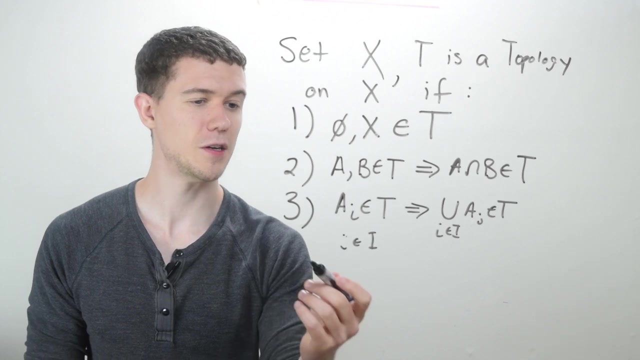 if you have any, any number of elements in t in your topology, any number of sets, their union is also in. t is also in the topology. So we say that t is closed under arbitrary unions And you'll see my notation here. I just said a sub i, So i is just like an indexing set. You can think of it. 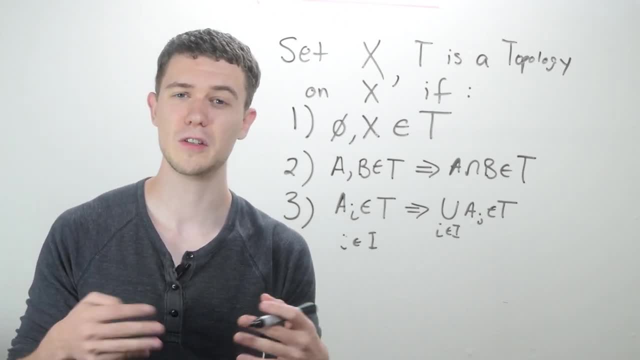 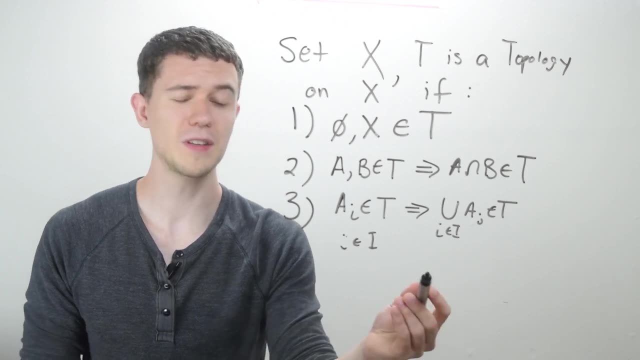 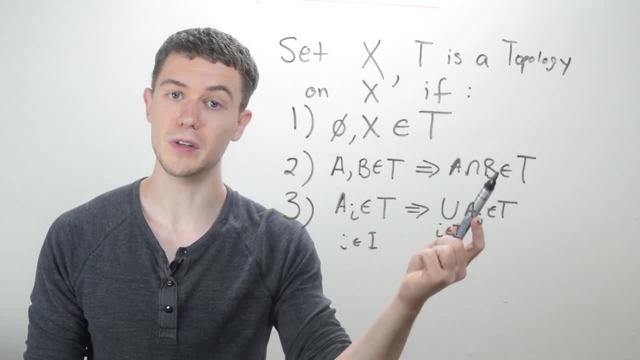 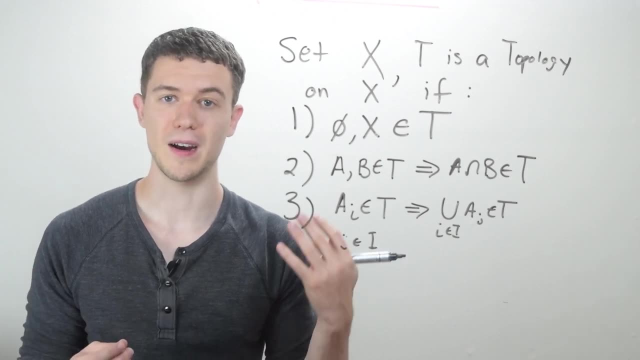 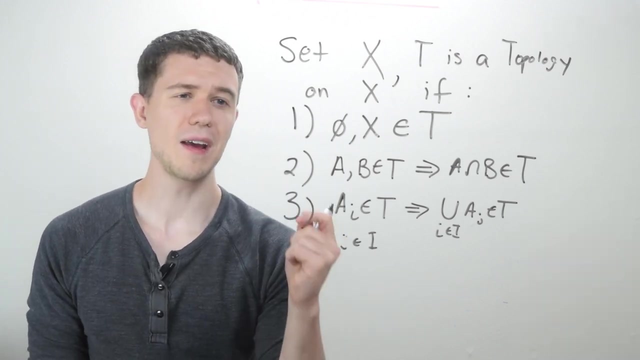 for each element in the topology. their union is also in the topology And union is just a mathematical way of saying both. So a union b would be everything from a and also everything from b. And so if you have these three things, if you have any set x, then t is a topology on x. 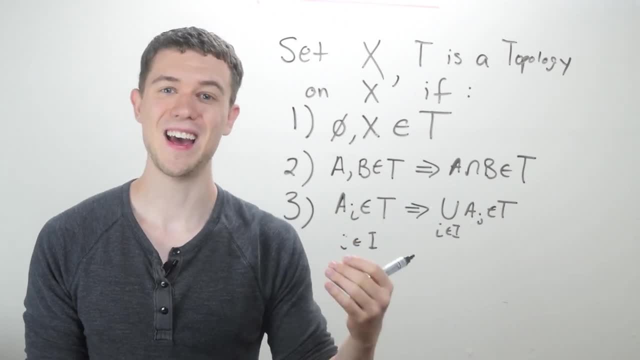 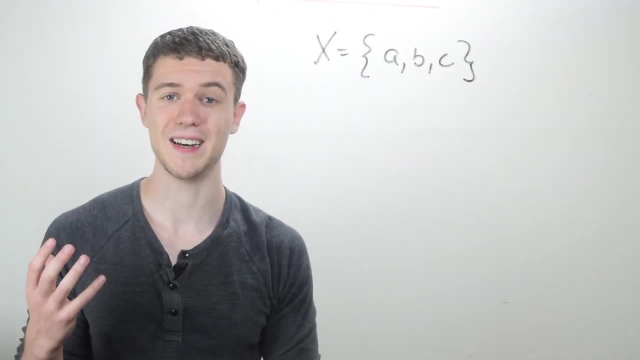 the set of sets, or rather a set of subsets of x, If it satisfies these three conditions. let's do this. Let's do an example. So here I have some arbitrary set x which has three elements, a, b and c, And let's create some topologies on x. 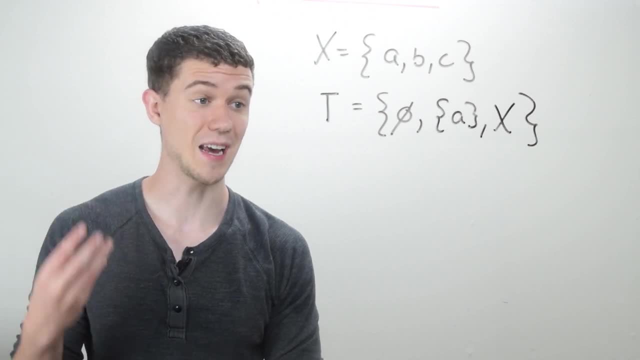 Okay, so now I've created this thing I've called t, that has the empty set, the singleton a, it's just the set containing only the element a, and also the set x itself. And is this a topology? Well, we have to check. So let's see Number one. 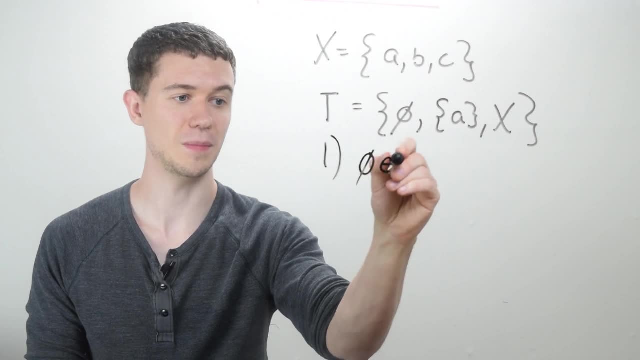 is the empty set a Number two is the empty set. a Number three is the empty set a Number four is the empty set in there? Well, yep, it's right there. So the empty set is in t That's good. 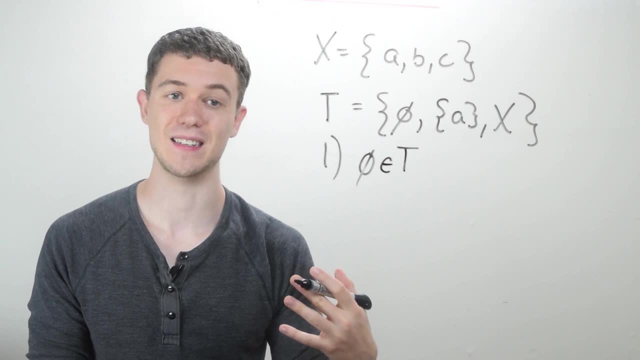 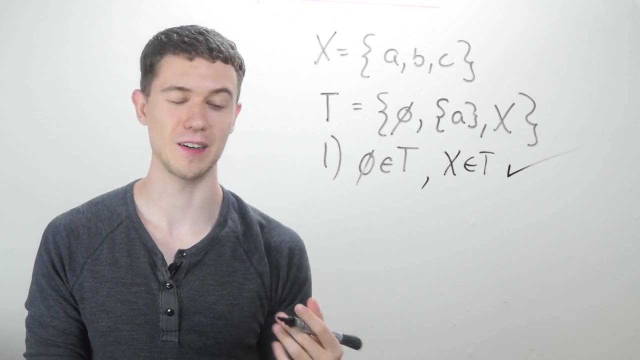 Is the entire set, the ambient set, x in t. Ah well, it's right there. So, yes, x is also in t. So that means, okay, good, Satisfied criterion number one. What's the second criterion? Well, 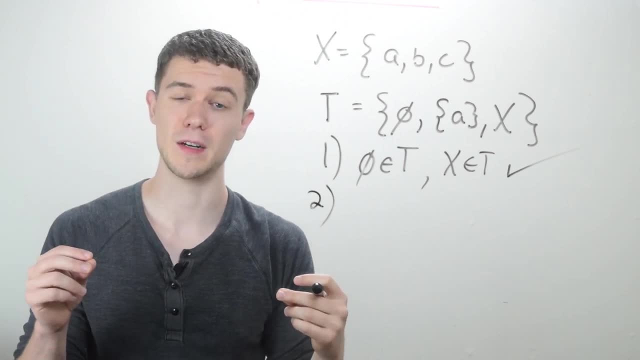 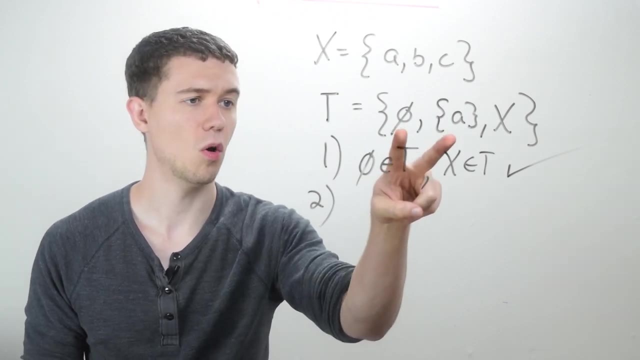 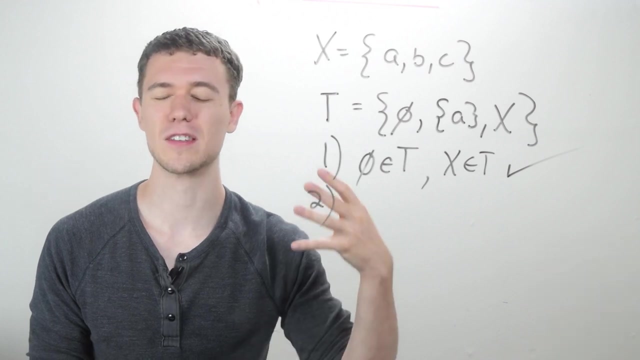 if I take any intersection of two elements in my topology, that also has to be an element of the topology. So let's intersect these things, Okay. well, what's the empty set? intersect any set? Well, it's the empty set, right, And that's sort of a set definition thing. 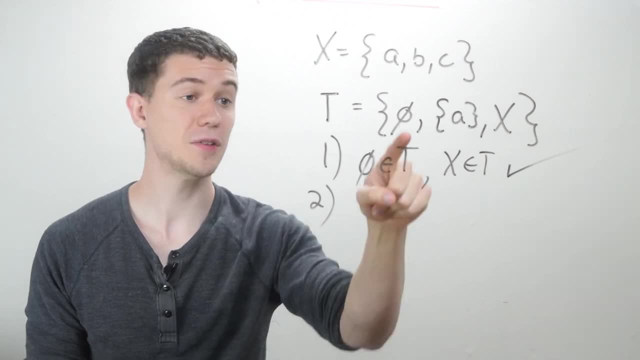 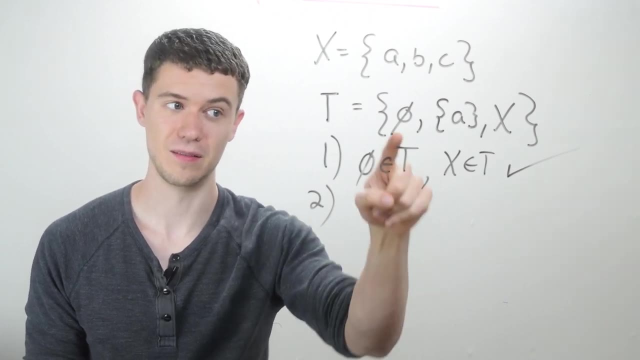 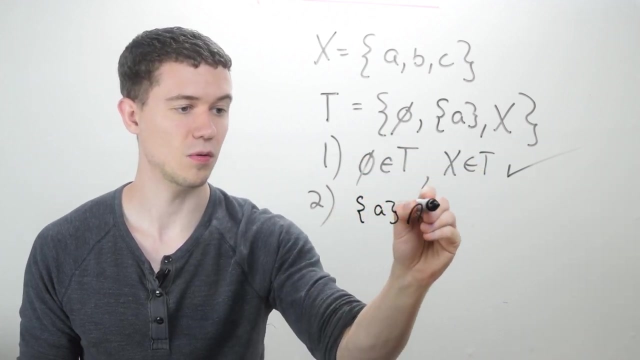 Anything intersected with the empty set is the empty set. If I intersect the set containing a or the set x with the empty set, I get the empty set, which is an element of t. So we're good with this. What happens if I intersect the set a with x? Well, a is an element of x, So the 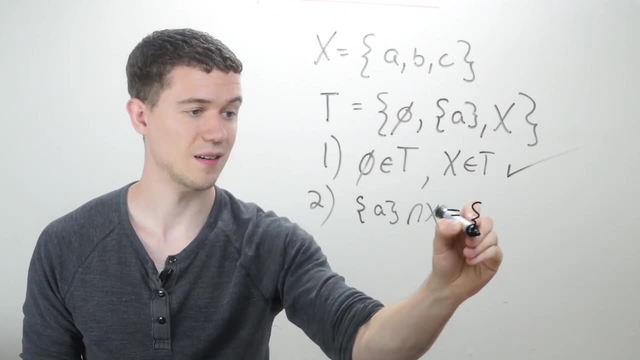 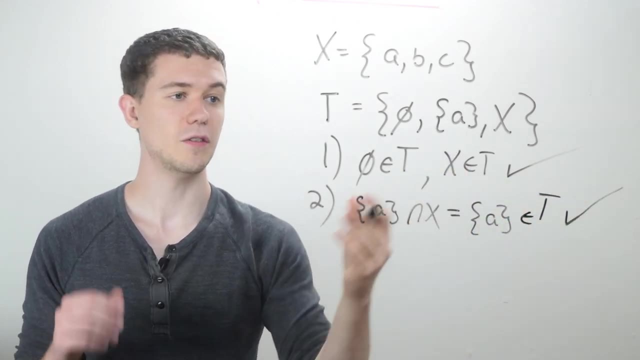 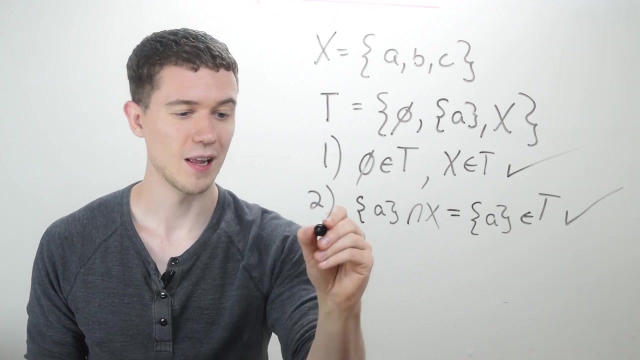 intersection of a and x is just a. Well, a is an element of our topology. So we can see here that no matter which way I intersect any two elements, they're an element in the set. So we've passed the second criterion for a topology. Let's check the third criterion. It's closed under arbitrary. 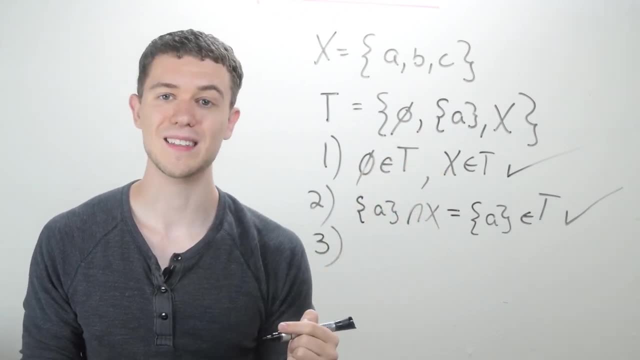 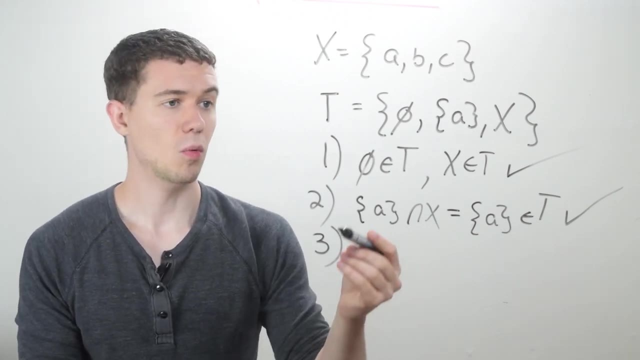 union. So I can take the union of any of these things and it should be in the set. Or I can take the union of all of them and it should be in the set. So let's see, Well, the union of the empty set with anything is just that thing. So, for example, 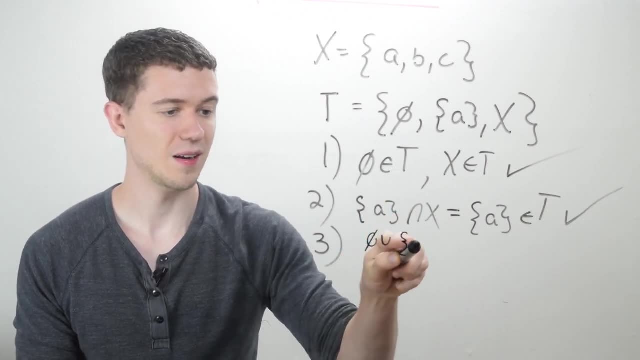 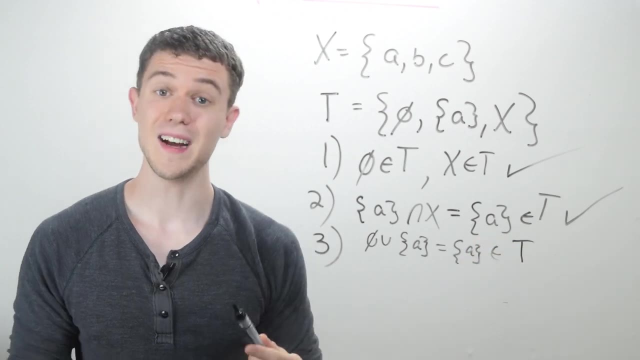 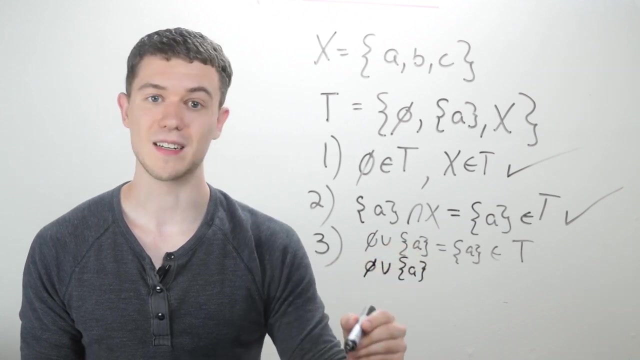 the union of the empty set and the set containing a is just the set containing a, which we said is an element of our topology. So that's a good check. What happens if I take the union of all three of these things? The empty set- union. the set containing a? union x. 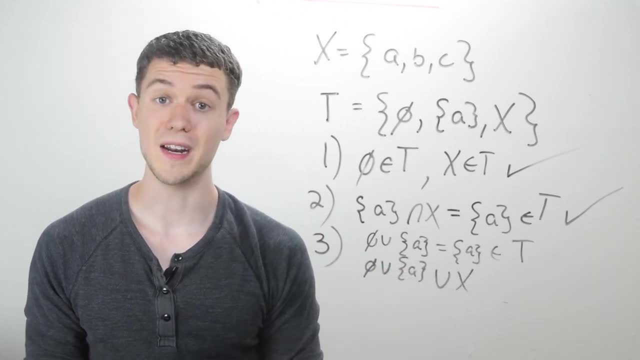 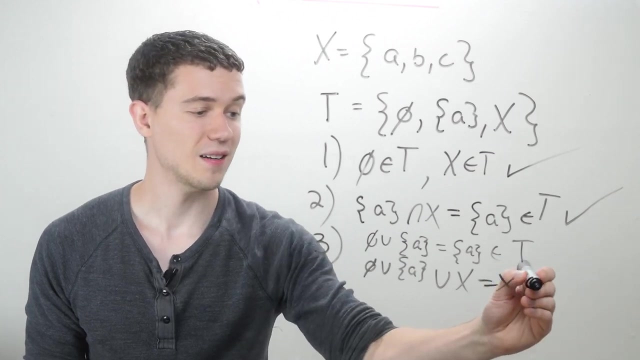 Well, the empty set union with anything is just that thing, And a is already an element of x, So x union, the set containing a is just x, right, Because a is a subset of x. So this is also in t by definition And you can check it's sort of. I could list all the ways to do this, But you can. 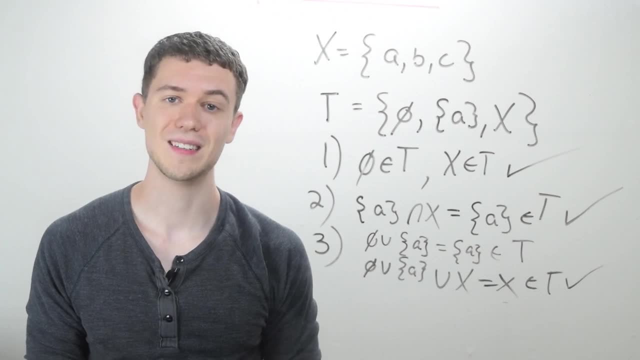 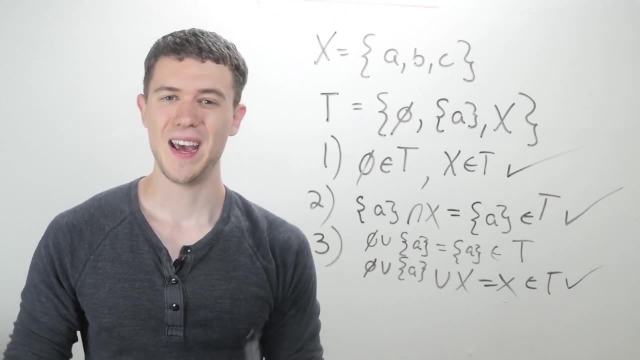 see that no matter how you union any of those things, that thing is still in t. So you can see that no matter how you union any of those things, that thing is still in t. So that's a good check, is still in the topology. And so those are the three criterion, And maybe this seems a little. 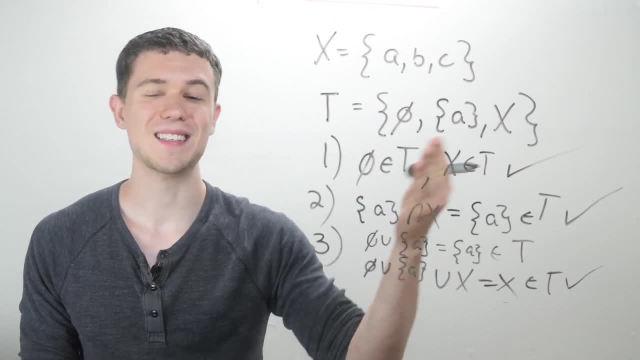 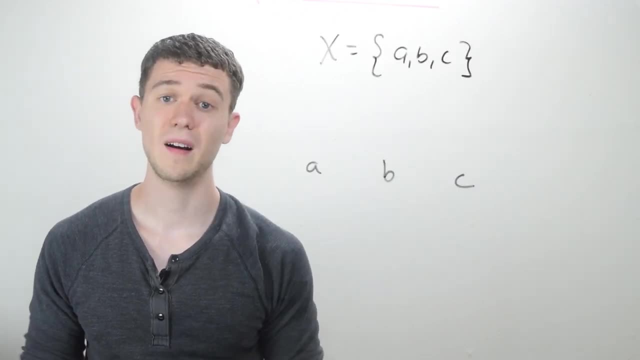 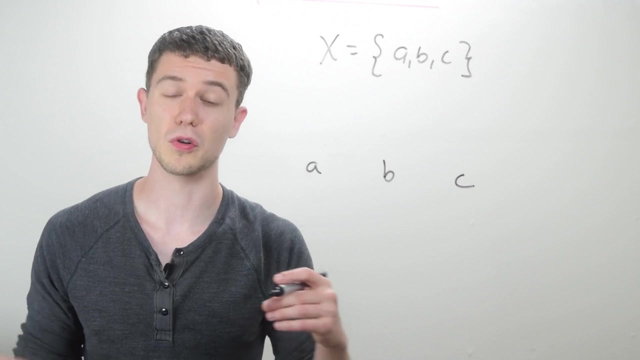 weird why we're doing this, But this we can see satisfies the three criterion for topology. So this T is a topology on the set x. Another way of looking at this is kind of by drawing a picture. So let's do the same sort of thing with A, B and C, So we'll just draw circles or ovals or 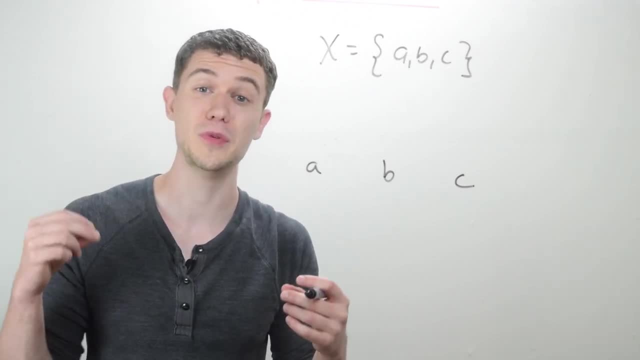 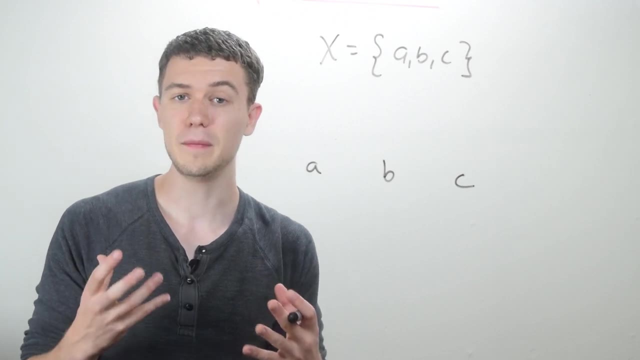 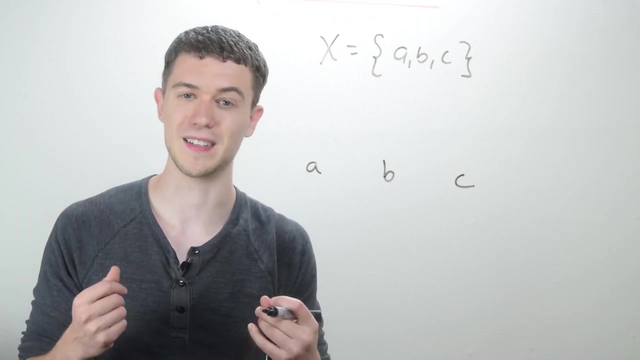 even rectangles around these things, And we'll let those open rectangles or circles be the elements of our topology. I mean, really, the elements of topologies are open sets. right, The elements of topologies are sets, We call them open sets, And so that's what I'm going to draw here. 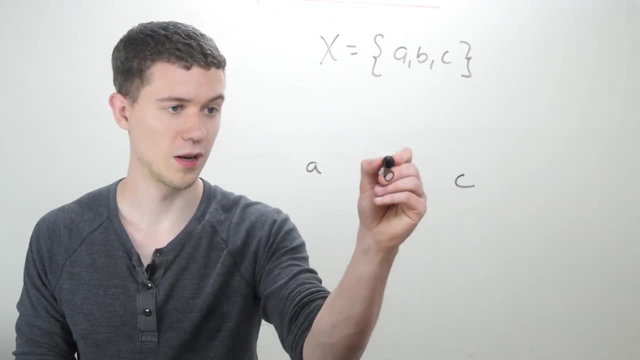 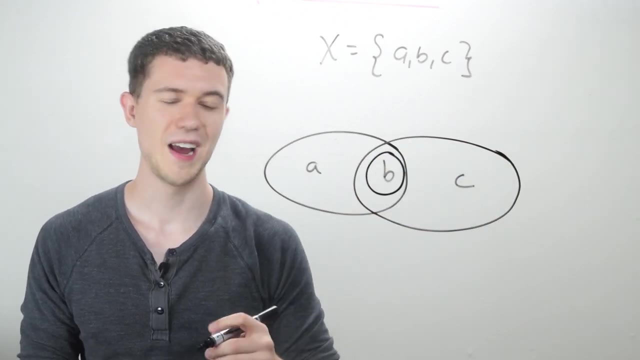 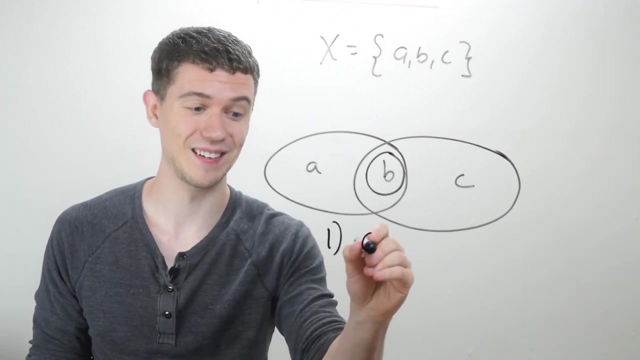 And we're going to decide if this is a topology or not. So I'm just going to draw. I'm going to draw some sets, some open sets. I'm going to draw it here And, okay, is this a topology? Well, let's see, The empty set is in here, right? So I'll call these open. 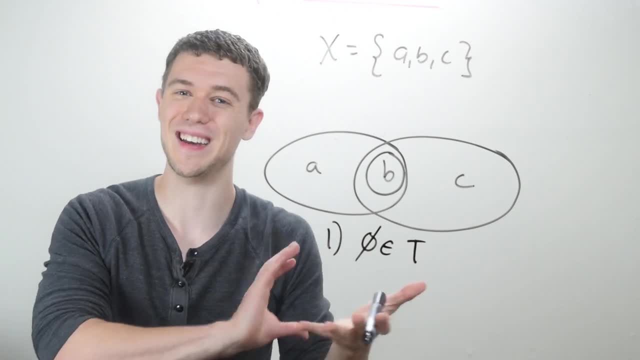 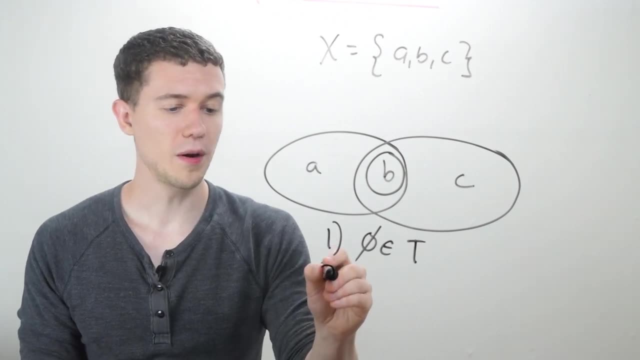 sets T, It's in there. because it's in there, we say vacuously: right, I didn't, I can't draw it, So it's in there. Well, what about? what about intersection? Do I have any of these circles? 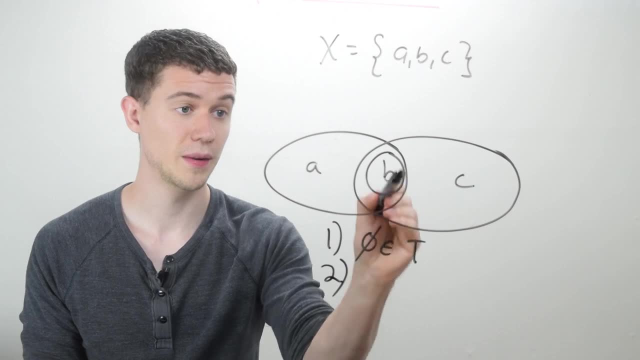 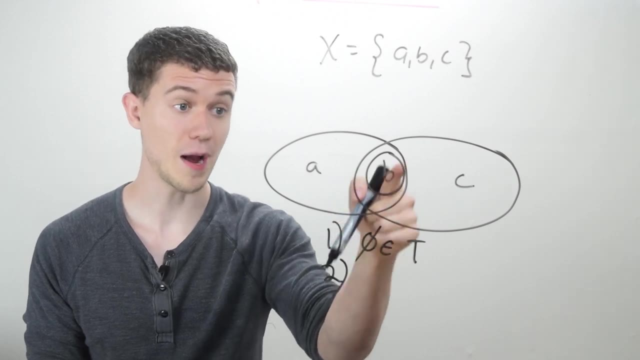 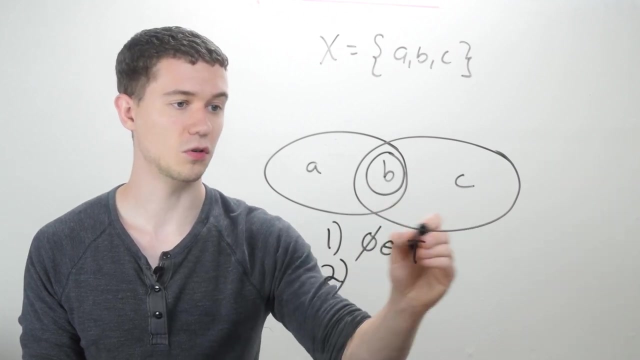 intersecting. Well, I've got this big circle intersecting with this big circle, and where is it? Where's their intersection? Where's there's overlap? Well, they overlap at B. Is there a circle around B? Yes, there is right. So the intersection of the circle containing BC. 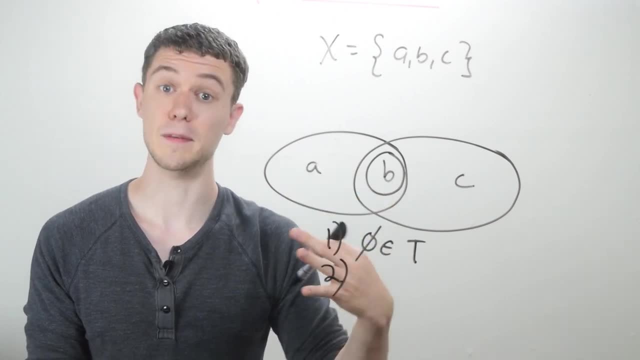 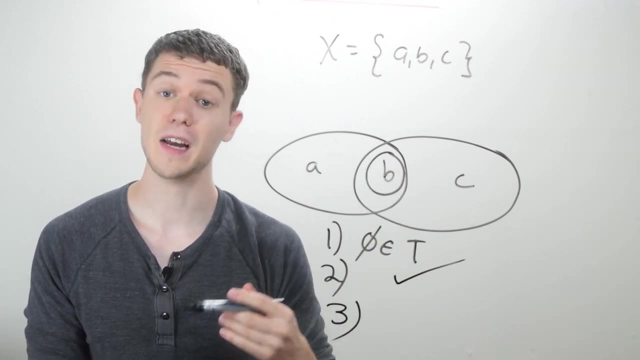 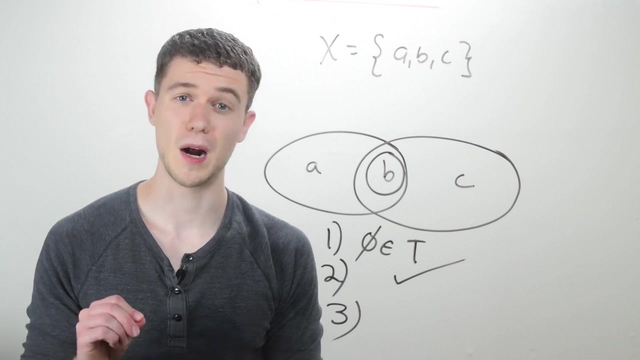 the intersection of the circle containing AB is B And there's a circle around B, So the second criterion holds And the third criterion is arbitrary unions. Well, if I try to union any of those, we run into a problem, And maybe you already recognize I kind of skipped over the very 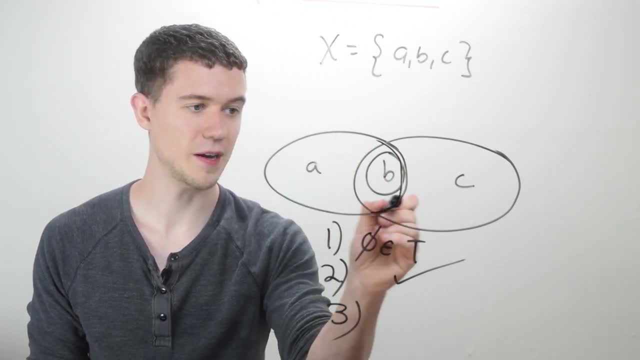 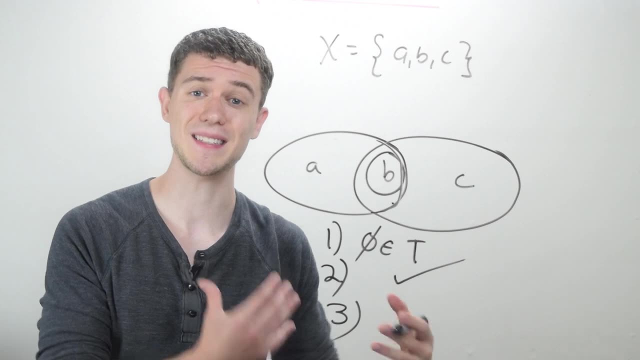 first thing, If I take this circle around A and B and I take this circle around B and C, why then I have a set containing AB and C, but I don't have any set containing AB and C. So the third failed. 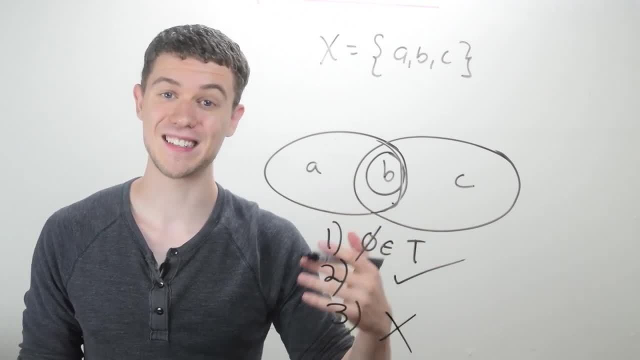 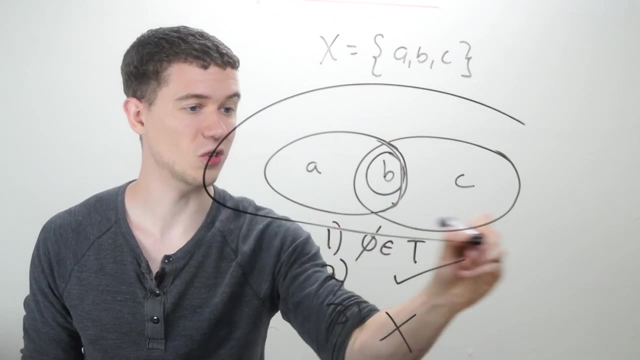 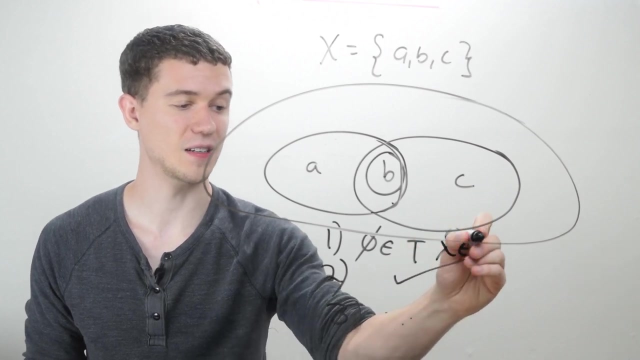 and actually the first failed too. if you remember what was the first criterion: x itself also has to be in the typology. For this to be a real topology, I need a big circle containing all of them. So if I include this big circle, then X is in the topology and we will be closed under arbitrary union.